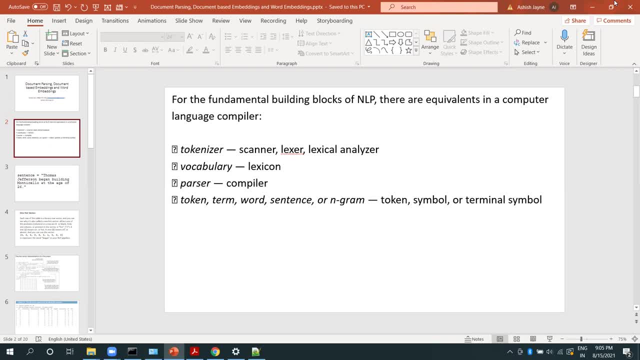 But if you take out characters and build your vocabulary on that, that will lead to huge memory use And most of the times people are okay with using words And the corresponding equivalent. if you have studied computer language compiler then you might be familiar with scanner like scanner or lexer. 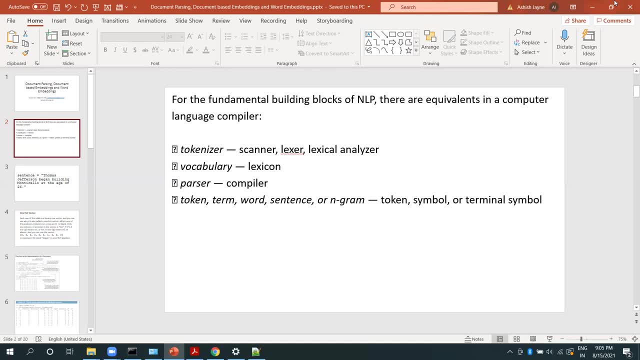 So scanner is basically that when you build, when you have to compile a code, you have to scan the code and you have to figure out if there are any syntax errors. And the result of that Tokenizer is that you get a vocabulary, you get words such as A and B or alpha, beta, gamma. 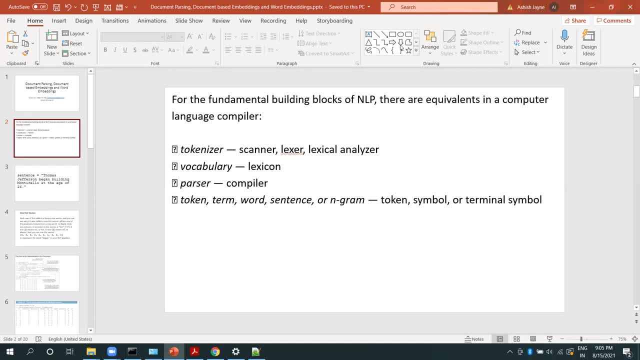 And what we get in a computer language compiler is lexicon, which is essentially tokens which are meaningful to the computer. Now, in NLP we have parser, in a computer language compiler we have compiler, and the whole process is that the outcome of this 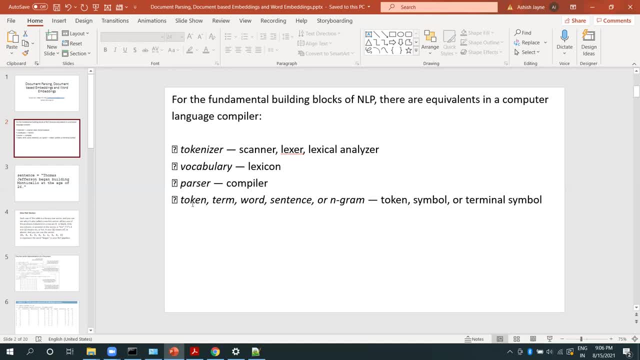 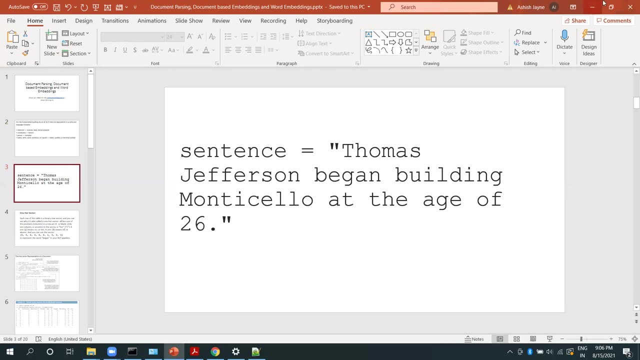 Tokenizer and building vocabulary and parser is that you get to understand the tokens in it, the terms, the words, the sentence in your natural language text. Now let's suppose this is a sentence given to us that Thomas Jefferson began building Monticello at the age of 26.. 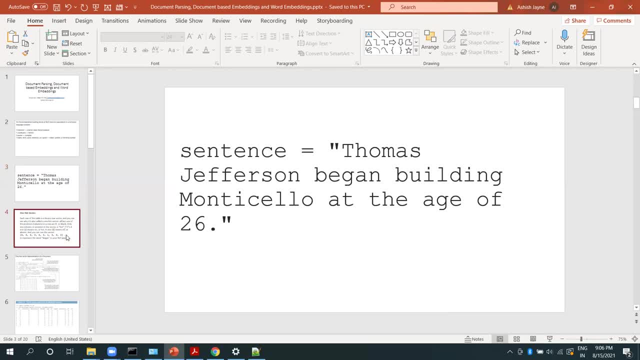 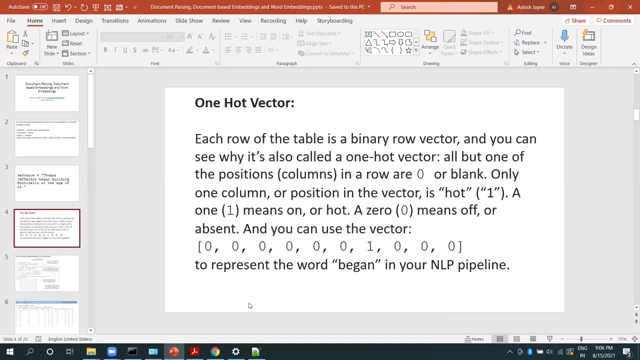 Now, if this sentence is given, we would work on it And Keep. I have presented the sentence over here because they're going to use it. going to be using it in that following slides. Now, this and this slide talks about one hot vector. 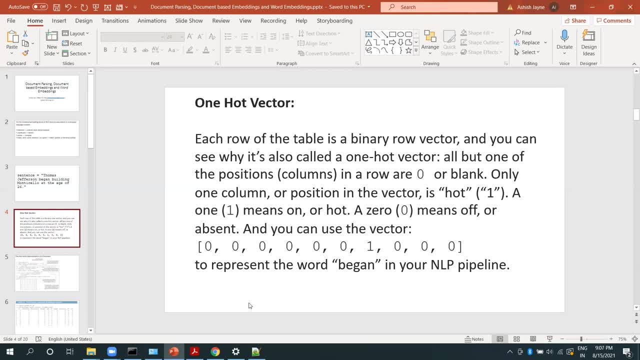 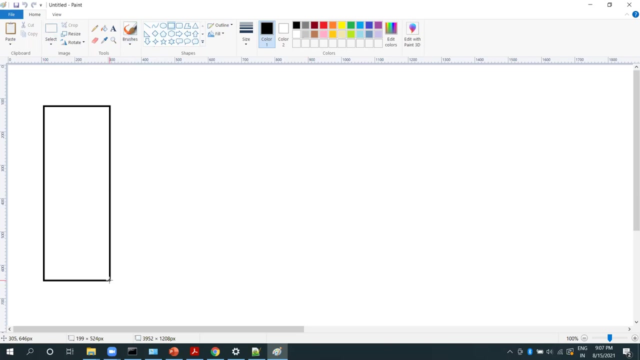 Are you familiar with one hot vector? If Yes or no, just a brief answer: No, Okay, so I'd explain. When you're given a text- let's say you are at open paint. instead of this, Let's say you have a column in which you are, you have values such as a, b, a, b. 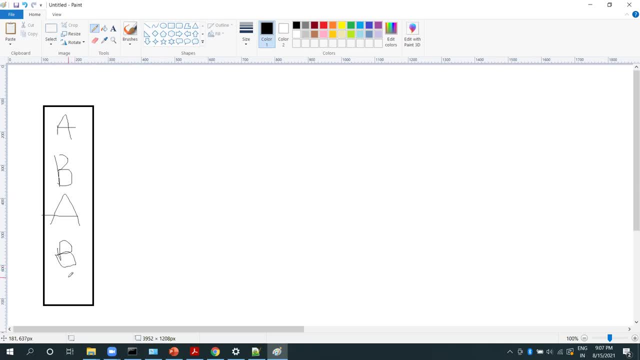 And then maybe We would just see and then be again. Now what would happen is that if you want to create a one hot vector from it, you would go this way: How many values do we have? One, two, three. 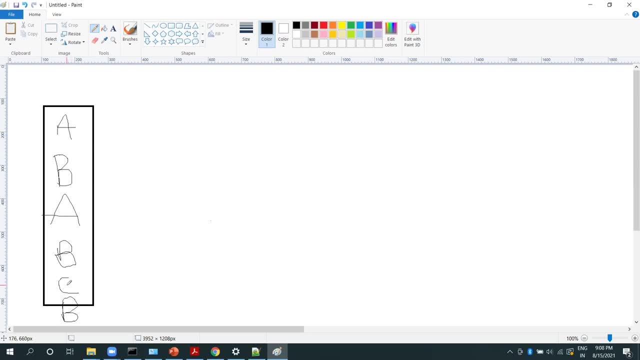 No, no, We have unique values: One, two and three unique values meaning how the set of all the values present in this column. Now, when we talk about creating a one hot vector From it, we essentially have to create three columns for each one of the variables. 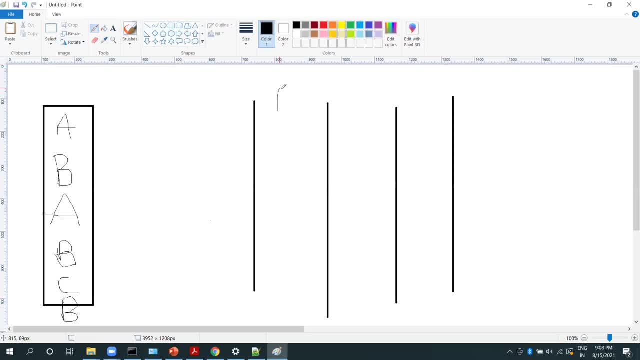 And we name them. we name them A, B and C. Now, when we name them A, B, C, then we start filling them. Do we have A here in this one, In this one, In this field? One second? 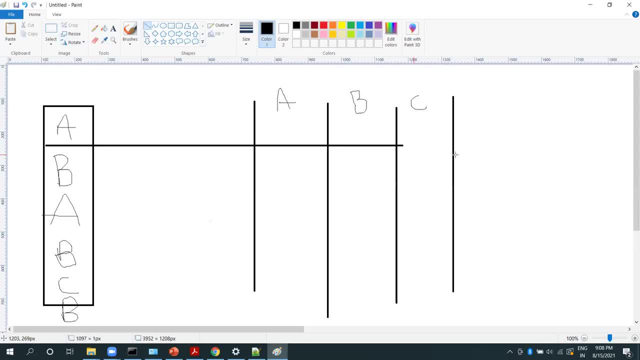 I'd also draw horizontal lines so that we don't confuse. Okay, Now to be. We have A here. Yes, we have A here. We would write one and zero in the others. If we do, we have B A here. 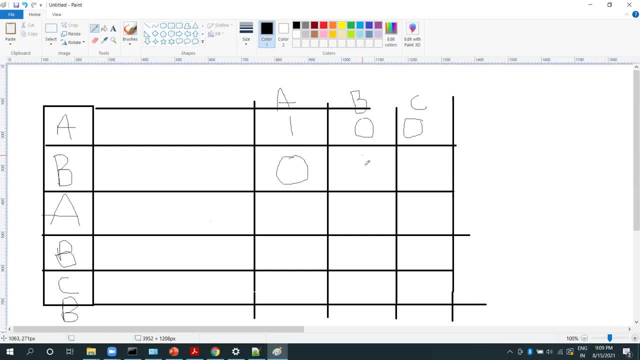 No, we don't have A here. Do we have B here? Yes, we have B here. Do we have C? No, Do we have A? Yes, B, No, C, No, B is there. So we put one on the one for B and zero for the rest. 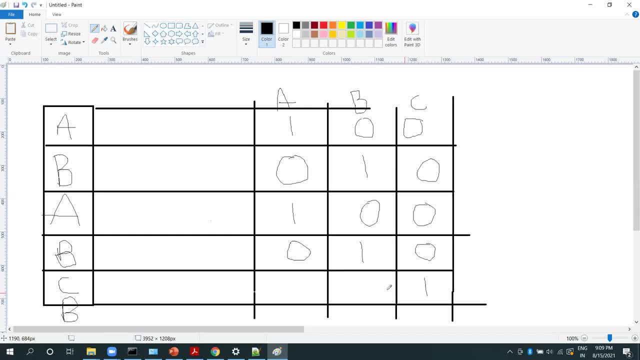 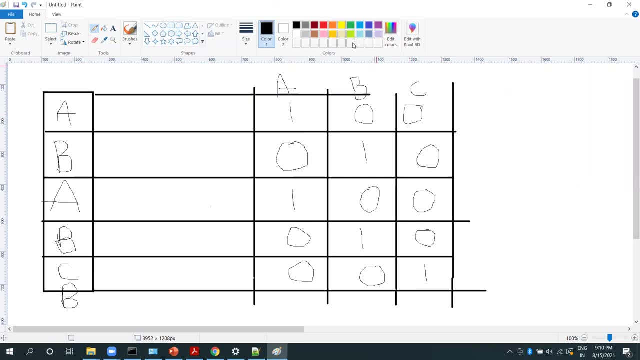 Similarly for C. we put one for C and zero for the rest. Now what is happening is we call this vector one hot vector, because only one value in the entire column is one and rest are zero. So this is basically one of the way to encode our incoming text into the form of zeros and ones, or that's how computers understanding. 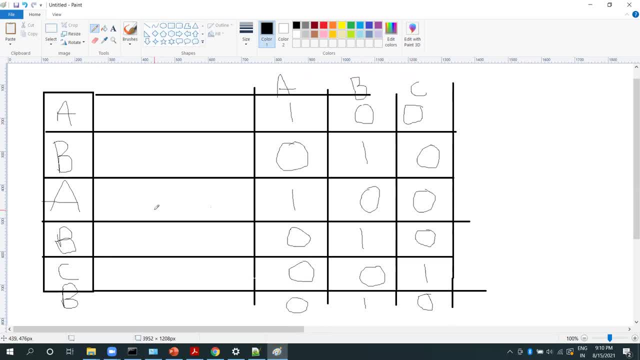 If you're given some text like this and you have to make them make it, make a computer understand that text, the first step you have to do is convert that natural language text into some kind of numbers. Okay, So let's say C. you want me to log into characters here? 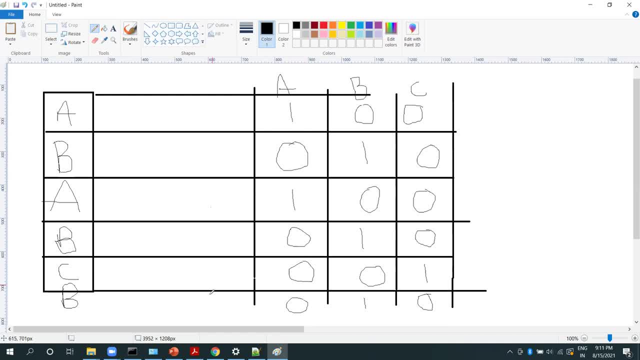 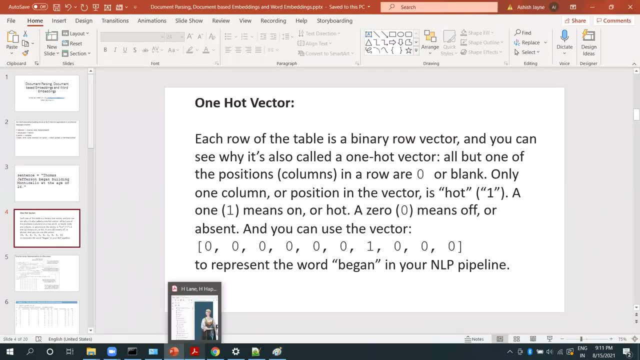 And you want to make a particular brand. sorry, the computer is tricking you that. this is not an action. and this is not an action, A character. a character is changing its name at random location: ital in… And you're looking at hexagons. 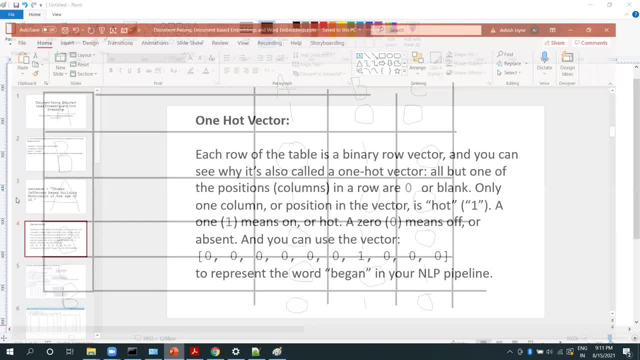 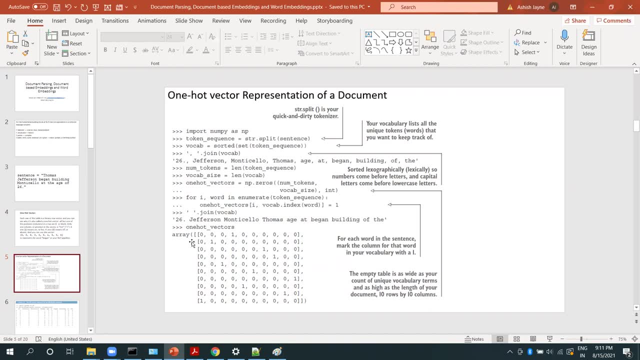 So, in this case, what you don't want, your renderіти are the view opinions right here. Right, Yes, it does. This is the shooter. He, Actually, he can see each one Akash plays in. Oh, we come back here. this is some code which is producing the one hot vector representation of 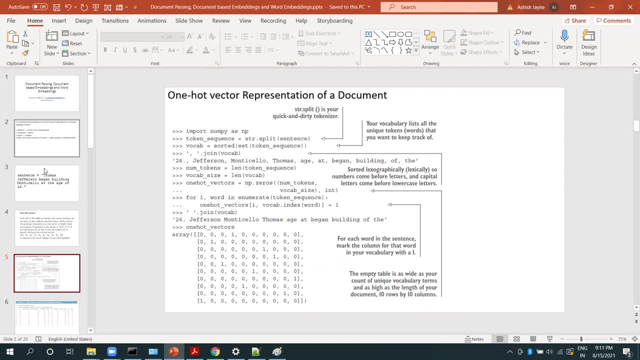 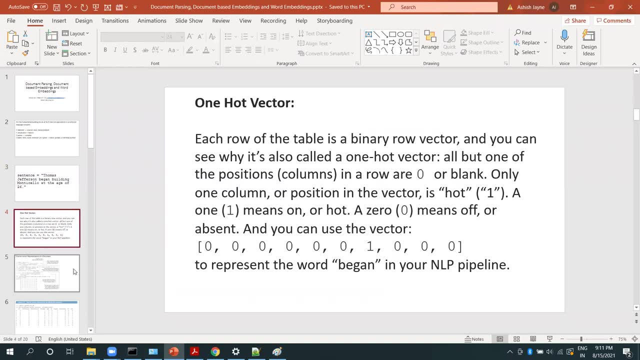 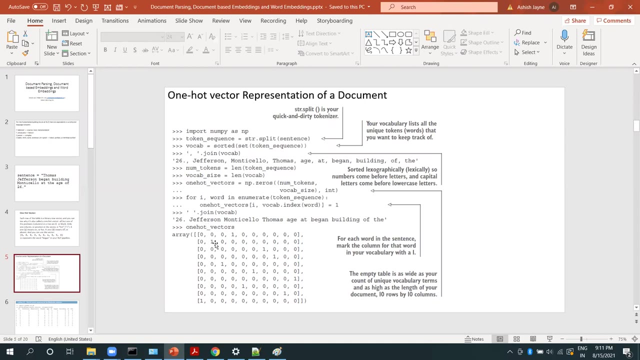 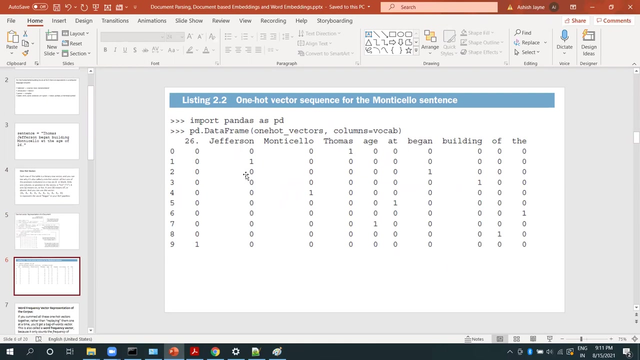 the sentence. the sentence is this: thomas jefferson began building monticello at the age of 26. now, what is happening here is it is trying to build a vocabulary by creating one hot vectors for the words, and the way it does is it has sorted the. uh, sorted the. 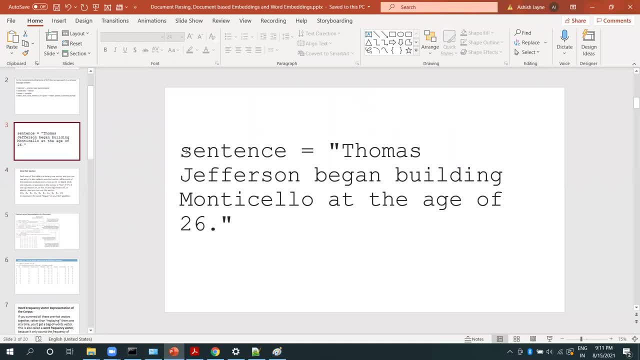 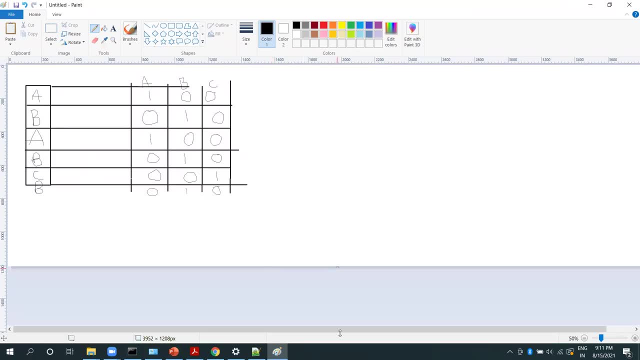 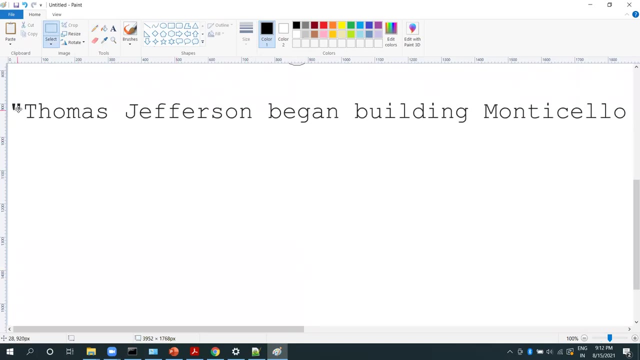 the sentences, sorted the words from the sentence. we have this over here now. if we go here and paste it here, then thomas jefferson began building monticello now. what words do we have here? monticello at the age of 26 right now? first step to building the one hot vector is that you have to sort the sort, the 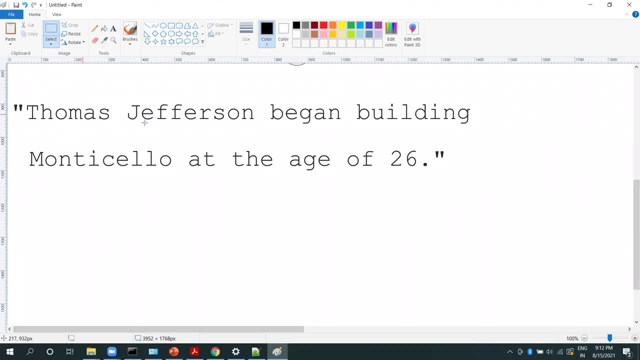 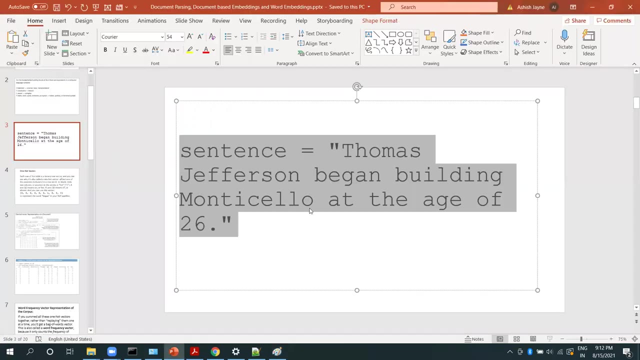 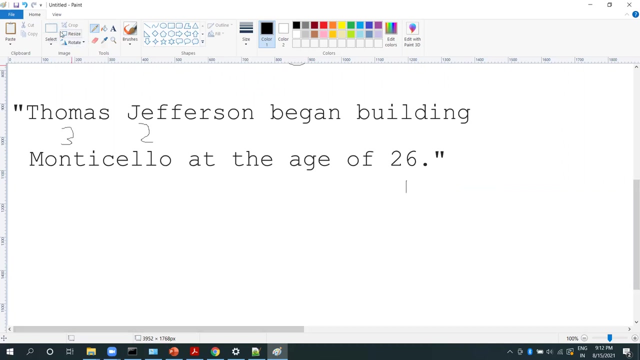 sentences: uh, sort the words in it. and the way it sorts word words is numbers are numbers comes first, then comes the capital letters, j, t, capital t, and then i think: okay, so not, not t, it's after j comes m, and this is how we. okay, this is how we. this is three. 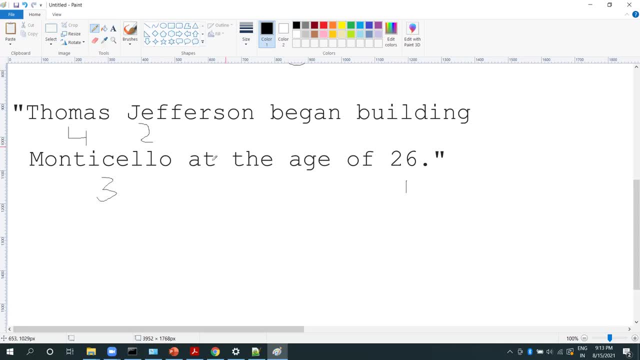 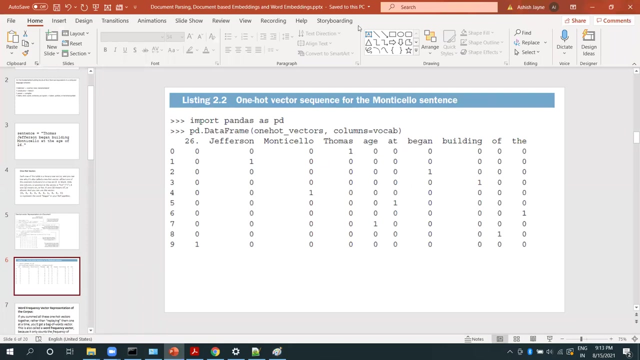 this is four, and then the small letters, which is pretty straight forward. page should come next age, yeah right, so so and so forth. okay, and six, so and so forth. essentially, it's created this matrix by creating this one hot vector. all of the code is present also on this page. you can refer to the. you can refer to the matrix which i had written in the usingheinli. 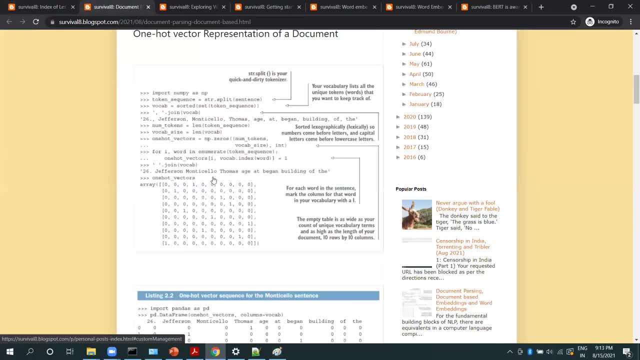 that is a formula for just um. so now you have these numbers which will appear on this page, which also would not mean you do not have to have these numbers. you just been usingheinli page. you can refer to it later, and this has been taken from this book. i shared the book with you. 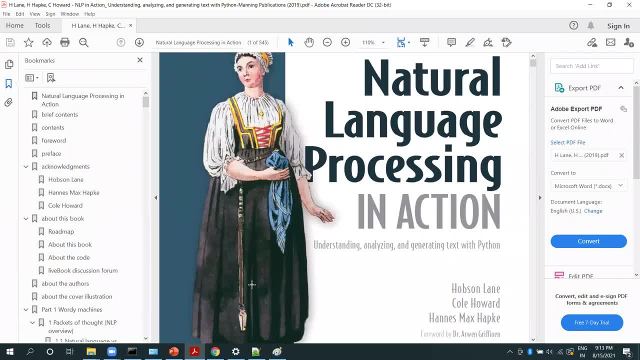 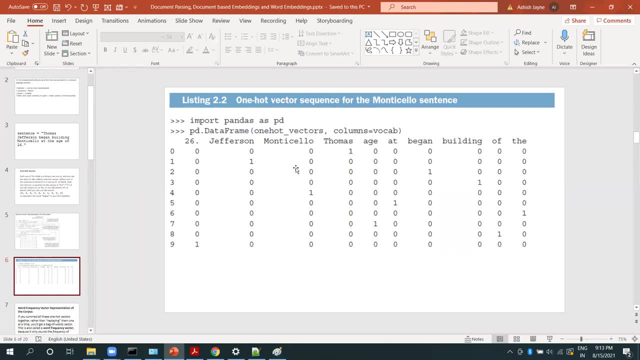 on later and you can go through it and this was for your understanding that how it creates one hot vectors. now what is happening is you are preserving the order. if we look at this line, it is saying first word is thomas and second word is jefferson. then next word is begin. it is: 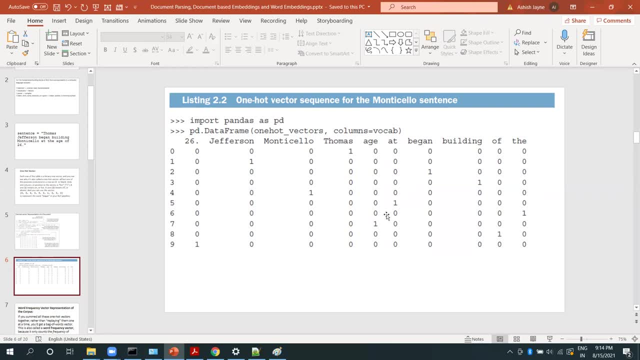 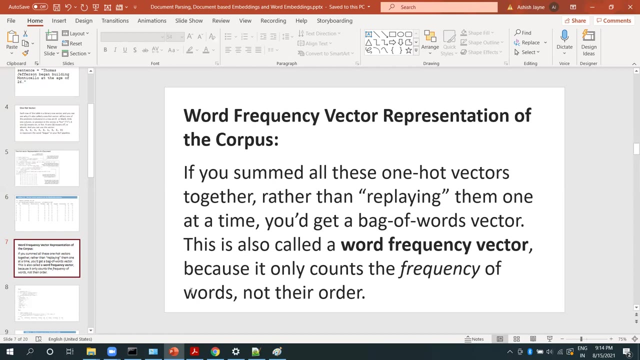 preserving the order of the words, but it is going to be huge, huge volumes of data if we store or our nlp text like this. now, the way to reduce that, the way to reduce that problem of overflowing memory and huge amounts of space requirement, we came up with the idea of bag of words vector, which is essentially we are only bothered about. 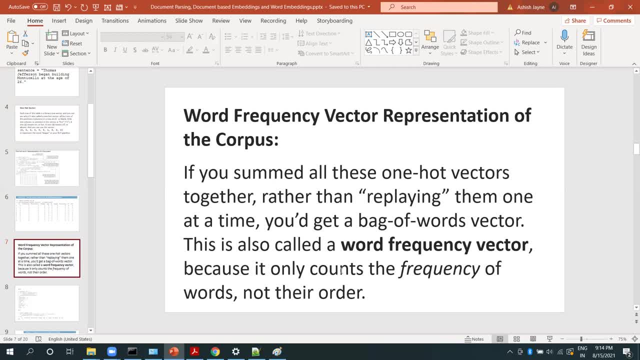 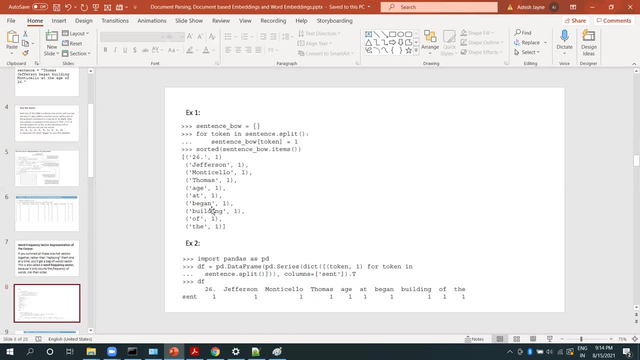 the word frequency, or frequency of the words, and not their order. so the next what we are going to create, the next vectors that we are going to create, will only consider the frequency of the words and not their order. now, if we do that, we only have to- uh, basically, if, if we do, 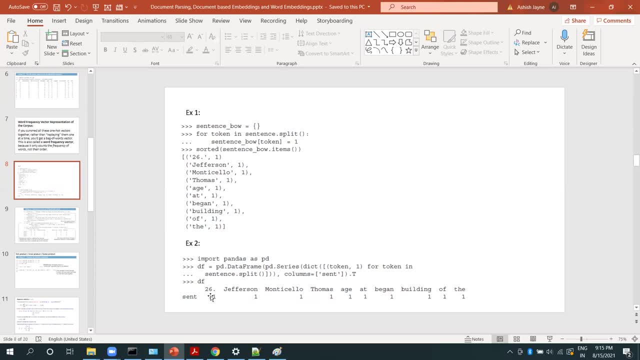 that we only have to uh, basically. if we do that, we only have to uh, basically, if. if we do that, we only have to uh, basically, if we do that, if we are presented only one sentence and we have all the words in it, we simply add one for every word. and if, in the representation bag of words, 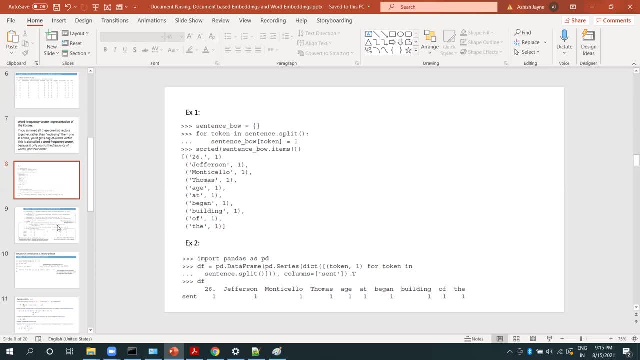 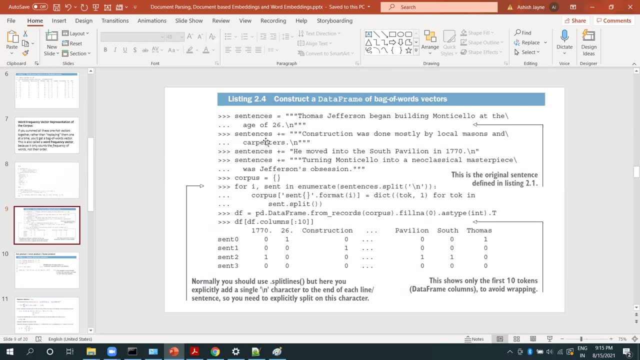 representation for that. that sentence would have all ones. but if we have more than one sentence like this one over here, let's say we have a couple of words here. thomas thomas jefferson. thomas jefferson, listing 2.7, one second. 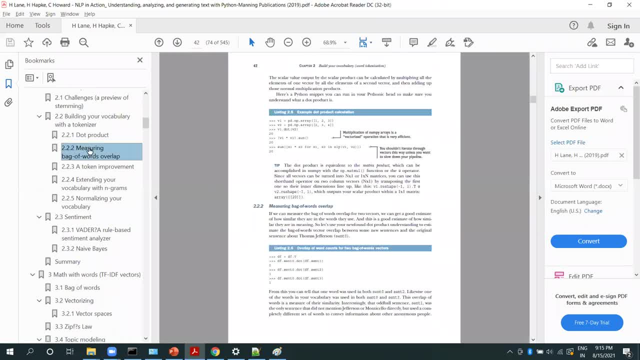 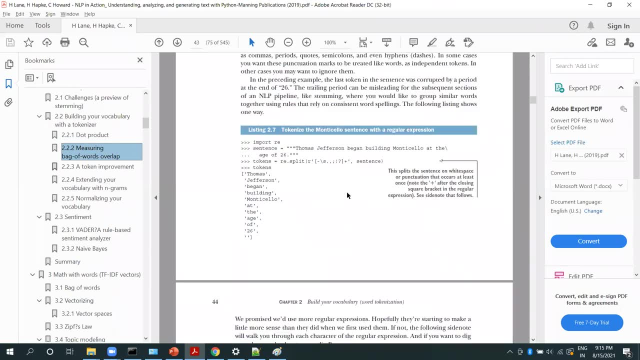 listing 2.7. one second listing 2.7. one second i'd i'd i'd open the listing. open the listing open. the listing 2.7: 2.7, 2.7, 2.5, 2.5, 2.5, 2.7. 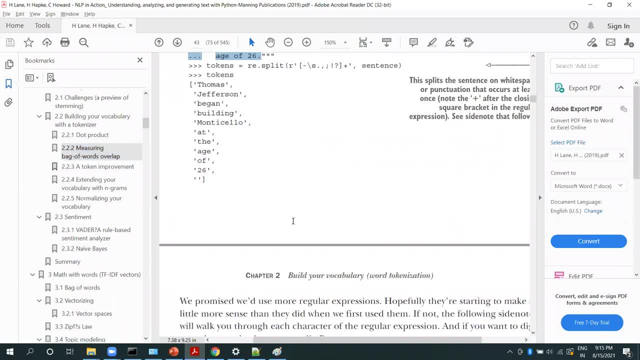 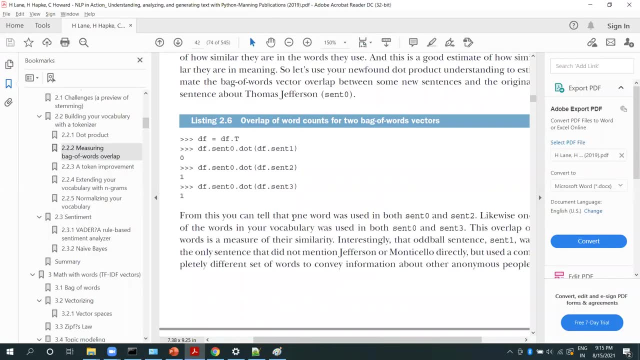 2.7, 2.7, 2.7, 2.7. so this is the first sentence, so this is the first sentence, so this is the first sentence, as we were seeing, as we were seeing, as we were seeing 2.4. okay, 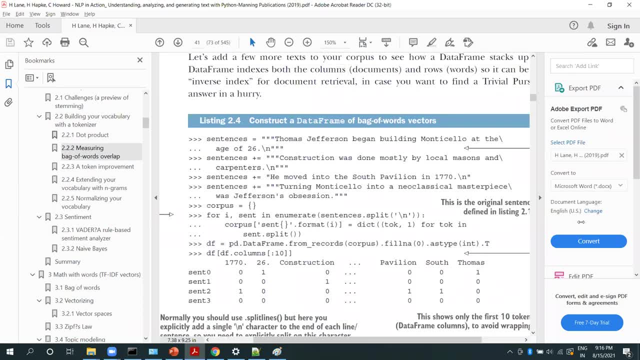 2.4, okay, 2.4, okay. so so this is the first sentence. so this is the first sentence, so this is the first sentence. so i'd explain, so i'd explain, so i'd explain. this is the first sentence. this is the first sentence. 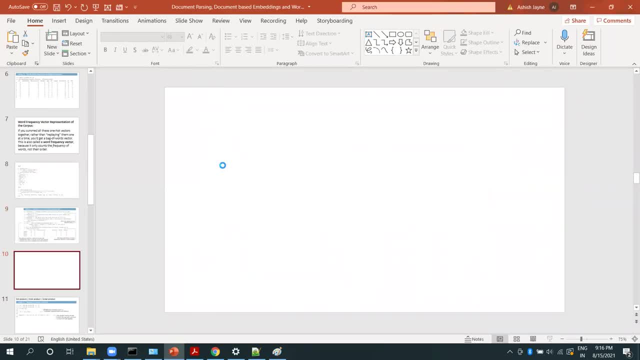 this is the first sentence. thomas jefferson. thomas jefferson. thomas jefferson: build began building monticello at the age. build began building monticello at the age. build began building monticello at the age of, of, of 26.. 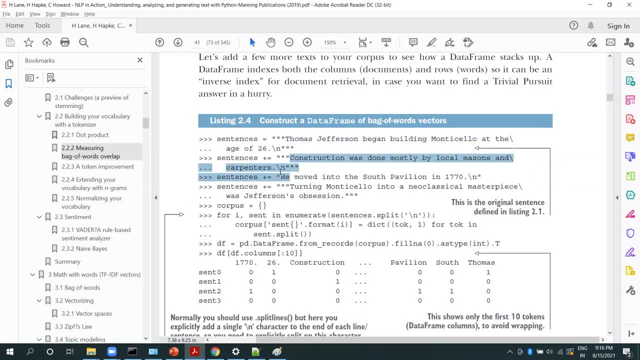 what is the second sentence construction? what is the second sentence construction? what is the second sentence construction? was done mostly by local mason. was done mostly by local mason. was done mostly by local mason, masons and carpenters. masons and carpenters. 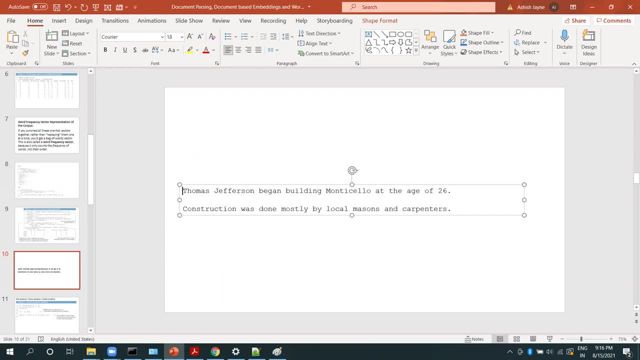 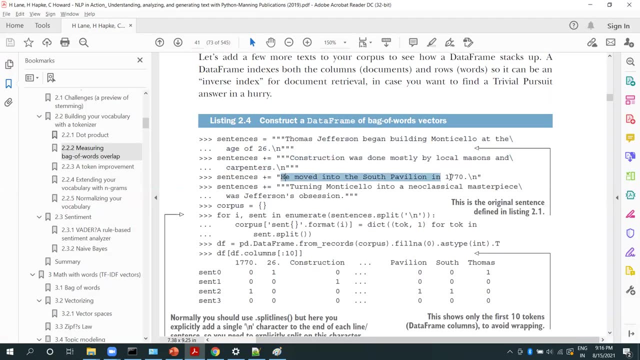 masons and carpenters. so this is the second sentence. third, is he moved to the south pavilion? third, is he moved to the south pavilion? third, is he moved to the south pavilion in 17 pavilion in 1770, in 17 pavilion in 1770? 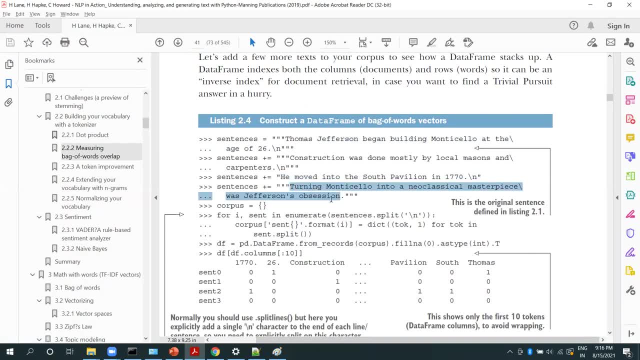 in 17 pavilion in 1770 and next last is turning monticello into and next last is turning monticello into and next last is turning monticello into a neoclassical masterpiece. was a neoclassical masterpiece. was a neoclassical masterpiece. was jefferson's obsession? now, if 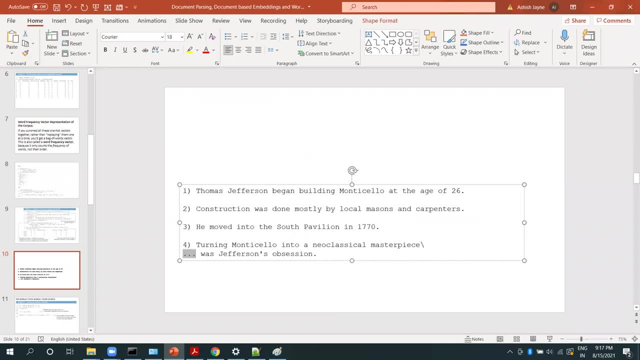 jefferson's obsession now. if jefferson's obsession now, if we look at it like we, we look at it like we, we look at it like we notice earlier notice earlier notice earlier: numbers come first right, numbers come first right, numbers come first right. and so what numbers do we have over? 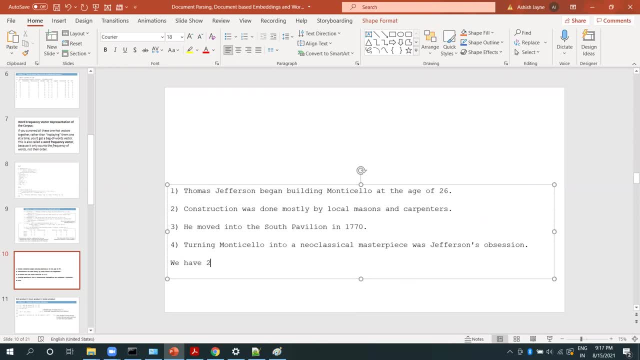 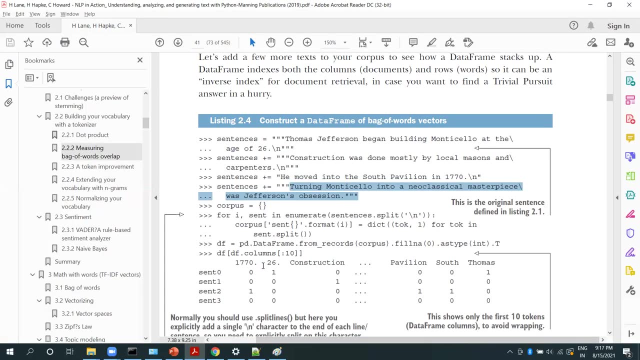 and so what numbers do we have over? and so what numbers do we have over here, here? here we have 26, and we have 26, and we have 26 and 17, 70.. 17, 70.. 17, 70.. and if we start building, 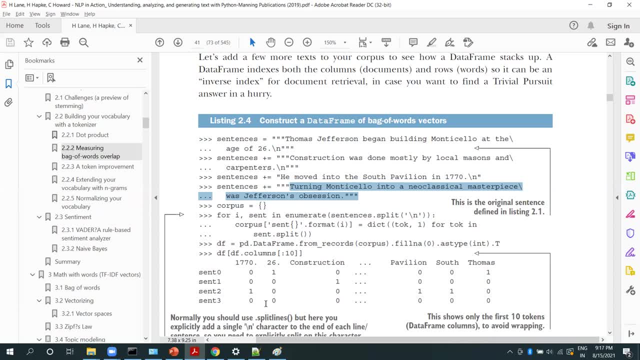 and if we start building, and if we start building bag of words for them, we would see that bag of words for them. we would see that bag of words for them. we would see that 26 is 26 is 26 is one for sentence zero, but 1770 is zero. 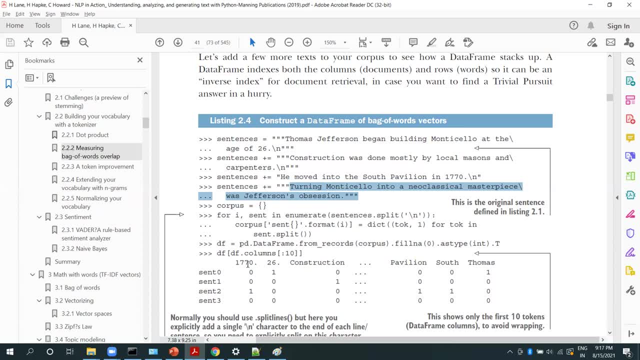 one for sentence zero, but 1770 is zero. one for sentence zero, but 1770 is zero. twenty twenty six is one for sentence. twenty twenty six is one for sentence. twenty twenty six is one for sentence, first sentence and 1770 for first first sentence and 1770 for first. 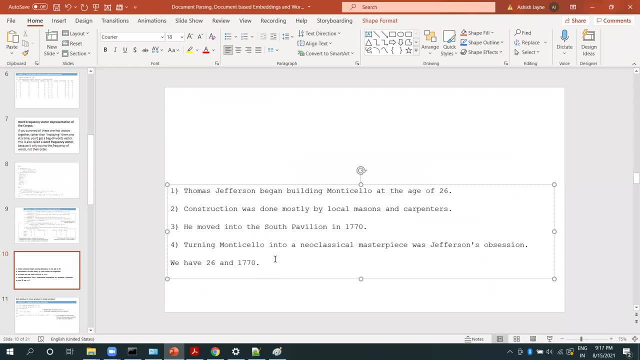 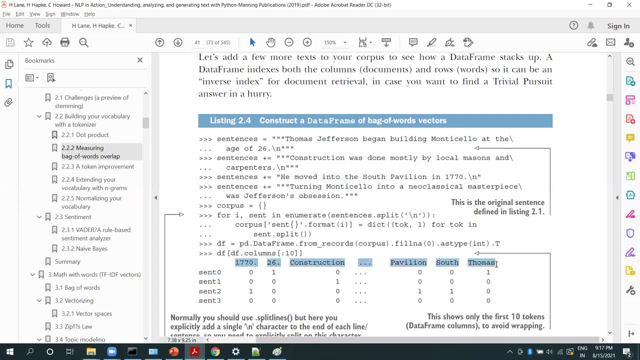 first sentence and 1770 for first sentence sentence sentence is zero. because is zero. because is zero. because 1770 is not here and how we got this. 1770 is not here and how we got this. 1770 is not here and how we got this for this x axis: this, how do, how did you? 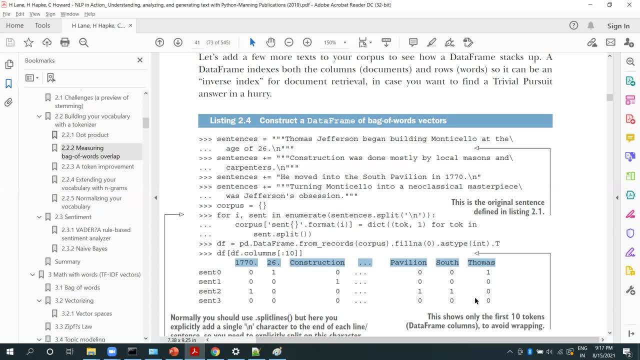 for this x axis this? how do, how did you for this x axis this? how do, how did you build this vocabulary? build this vocabulary? build this vocabulary is by parsing, so what happens? you is by parsing, so what happens. you is by parsing, so what happens? you tokenize, you pick every word in it, thomas. 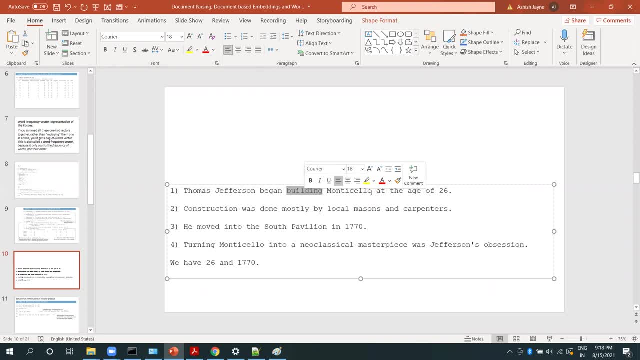 tokenize you pick every word in it. thomas. tokenize you pick every word in it: thomas. is there Jefferson is there began? is? is there? Jefferson is there began? is? is there Jefferson is there began? is there building? is there Monticello at the there building? is there Monticello at the? 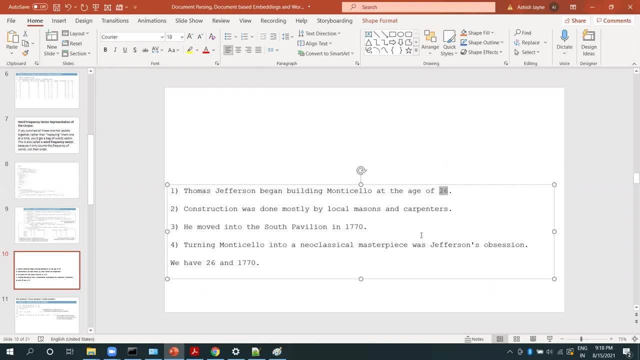 there building? is there Monticello at? the age is there of? is there 26? is there? age is there of? is there 26? is there? age is there of? is there 26? is there? tokenization gives you the words you. tokenization gives you the words you. 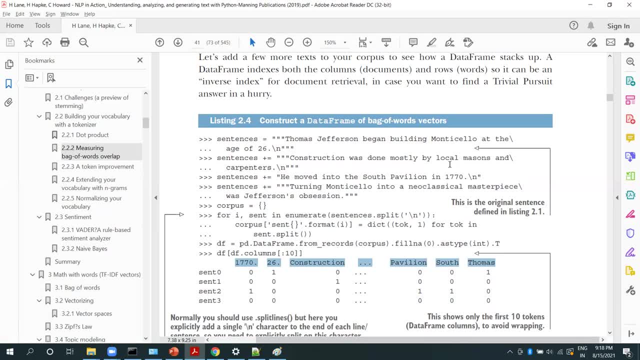 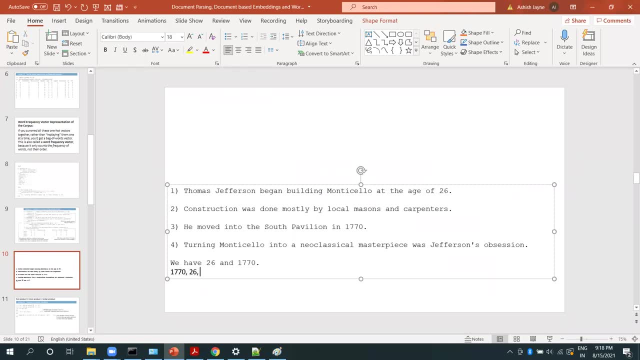 tokenization gives you the words: you sort them, you put them in order, sort them. you put them in order, sort them. you put them in order: 1770, 26 construction. 1770, 26 construction. 1770, 26 construction. so i'd write it down: 1770. 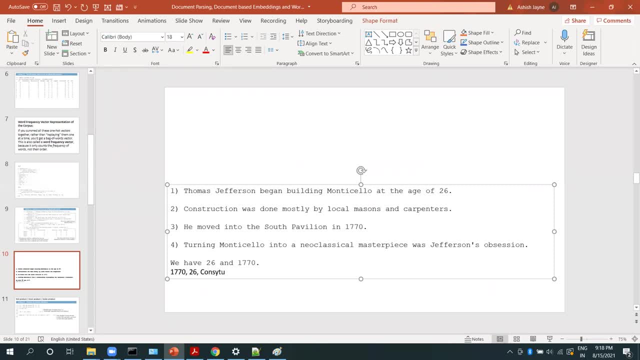 so i'd write it down 1770. so i'd write it down 1770: 26 construction, 26 construction, 26 construction. can you tell me which is going to be? can you tell me which is going to be? can you tell me which is going to be the next word? 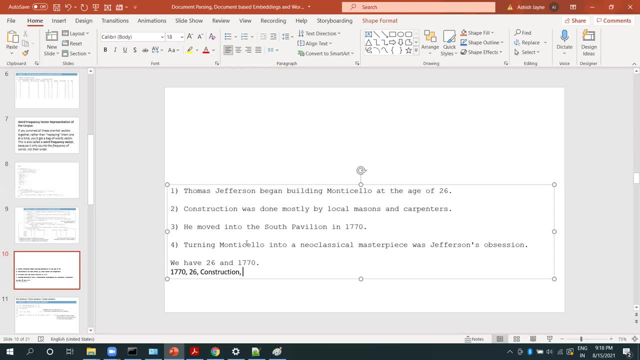 the next word, the next word, some word with capital, some word with capital, some word with capital letter. i think it's gonna be letter. i think it's gonna be letter. i think it's gonna be jefferson jklm. yeah, jefferson jklm, yeah. 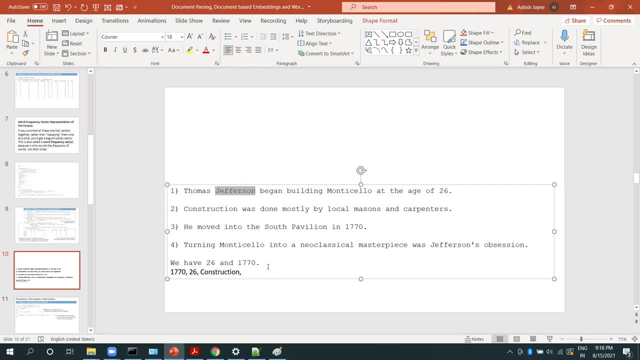 jefferson, jklm. yeah, it's gonna be jefferson. it's gonna be jefferson. it's gonna be jefferson. yes, i think it's gonna be key. so this is the kind of this is. so this is the kind of this is. 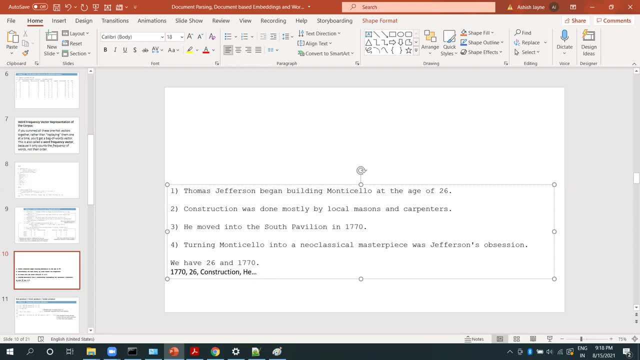 so this is the kind of this is sort of so this is the kind of this is sort of how, how, how, uh, the vectors are built and we can uh the vectors are built and we can uh the vectors are built and we can take down the last from here. pavilion. 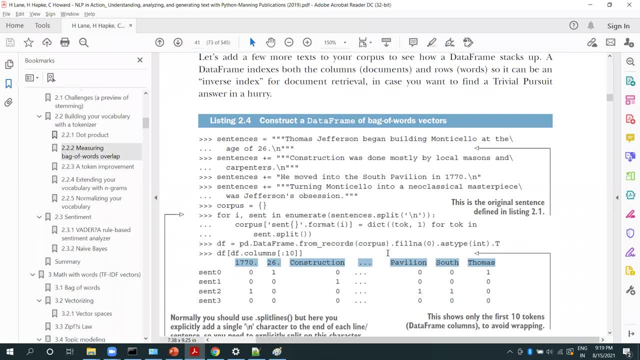 take down the last from here, pavilion. take down the last from here, pavilion. south, south, south, thomas, i think it. he has this author has thomas. i think it, he has. this author has thomas. i think it, he has. this author has only picked out the capital words. 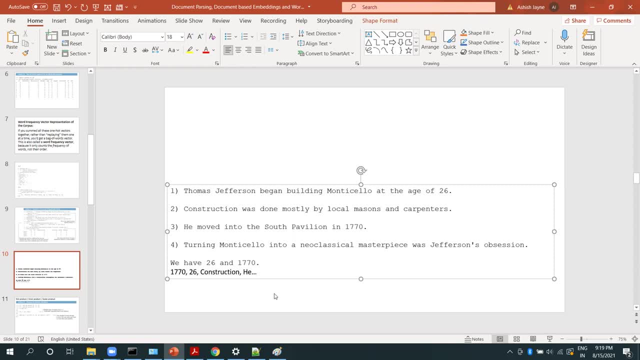 only picked out the capital words, only picked out the capital words and not the um and not the um and not the um, not the small words, not the small words, not the small words. so so so, twin building, twin building, twin building, the vocabulary now. the vocabulary now. 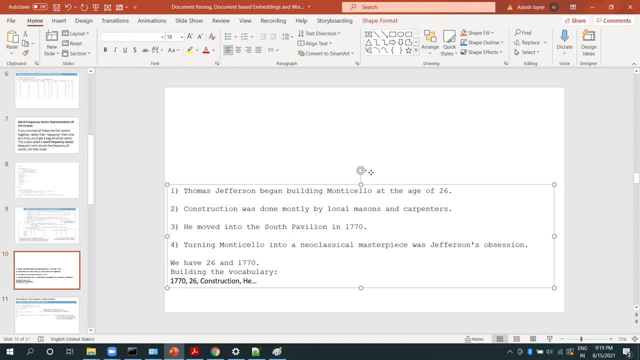 the vocabulary now, once we are, once we are doing that. once we are once we are doing that, once we are once we are doing that, uh, uh, uh. we have to construct a matrix of this. we have to construct a matrix of this. we have to construct a matrix of this form. 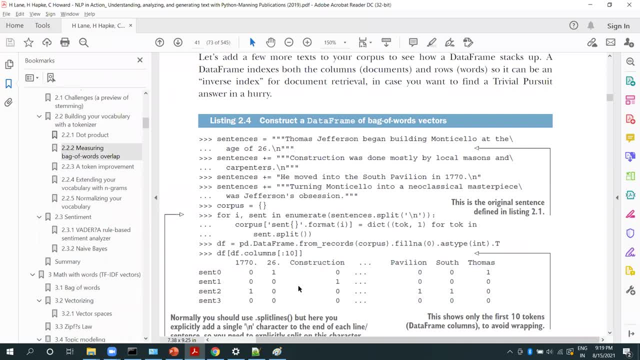 form, form: zeros and ones. so for every word in zeros and ones. so for every word in zeros and ones. so for every word in that sentence, that sentence, that sentence, we put a one for the column, we put a one for the column, we put a one for the column corresponding to that word. this gives: 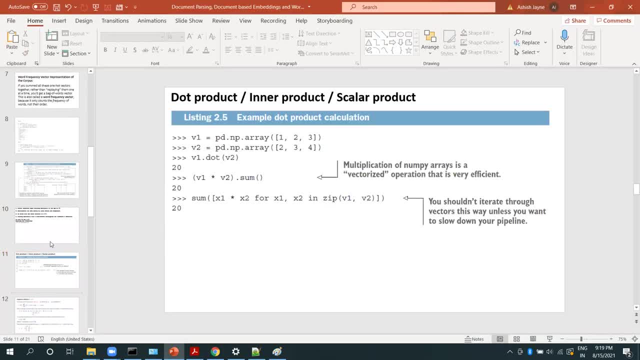 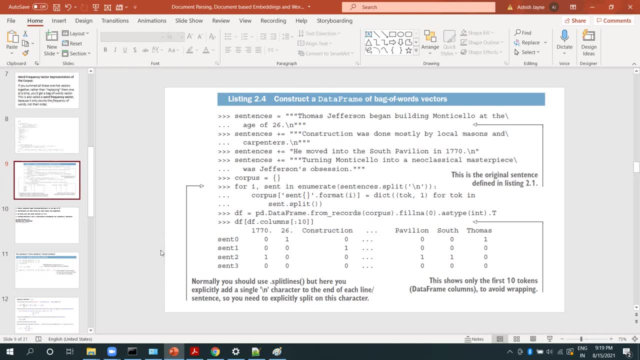 corresponding to that word. this gives. corresponding to that word. this gives you the one hot wick. you the one hot wick, you the one hot wick. oh no, no, uh. this bag of words model. oh no, no, uh. this bag of words model. oh no, no, uh, this bag of words model for your. 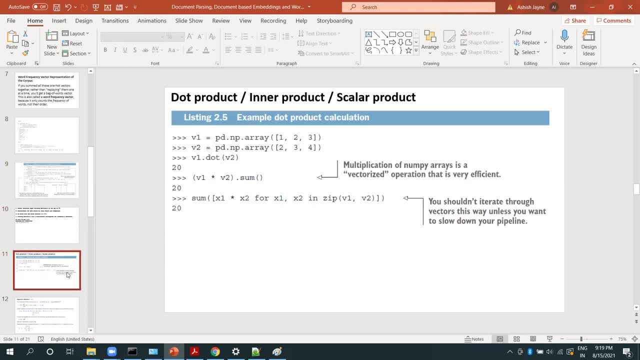 bag of words vector for your sentences. bag of words vector for your sentences. bag of words vector for your sentences, and, and. and this is basically just just for. this is basically just just for. this is basically just just for additional information. dot product is a additional information. dot product is a. 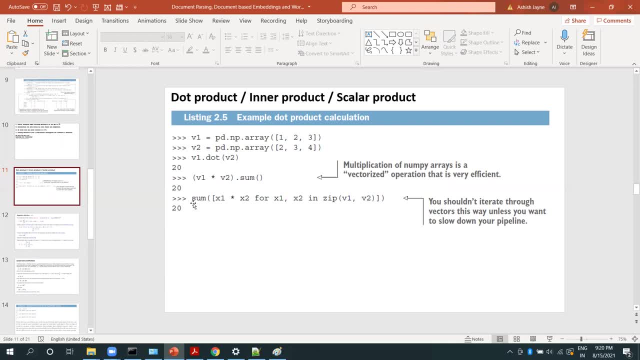 additional information. dot product is a very important operation, very important operation, very important operation in nlp. this is one of the matrix in nlp. this is one of the matrix in nlp. this is one of the matrix operations that i found, operations that i found, operations that i found in one of the pages in the book and you. 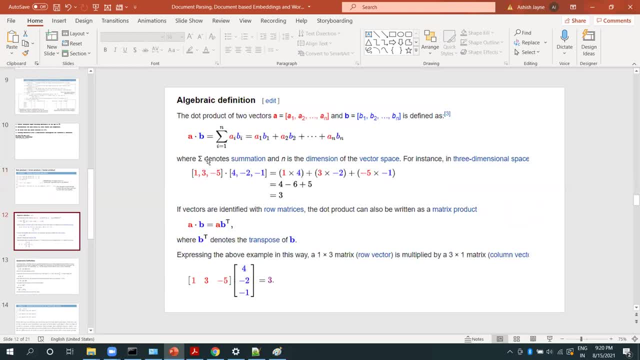 in one of the pages in the book and you in one of the pages in the book and you can just remember that, can just remember that, can just remember that algebraic definition of this is if you're algebraic. definition of this is if you're algebraic definition of this is if you're given a dot p and you know the values. 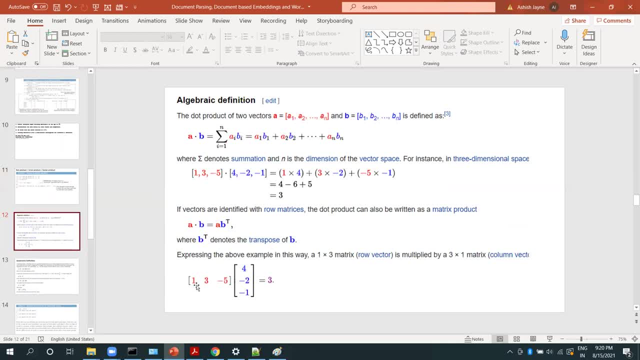 given a dot p and you know the values given a dot p and you know the values: a1, b1, a2, b2, a1, b1, a2, b2, a1, b1, a2, b2, it's sort of like this: a1, b1. 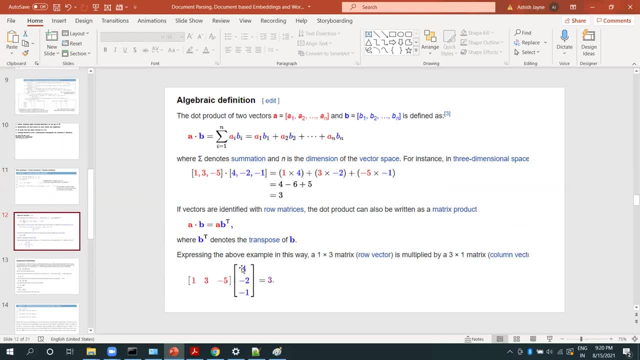 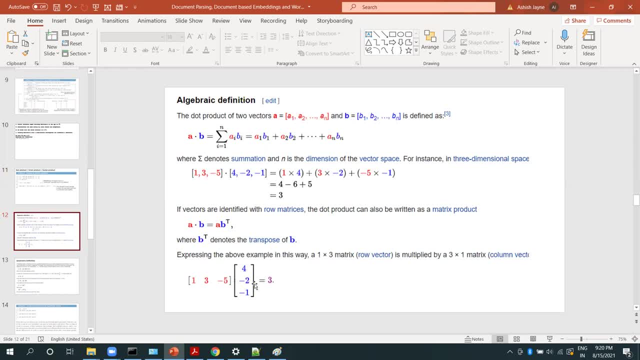 a1, a2, a3, a1, a2, a3, b1, b2, b3, then you multiply them. this is b1, b2, b3, then you multiply them. this is b1, b2, b3, then you multiply them. this is the dot product of these two. 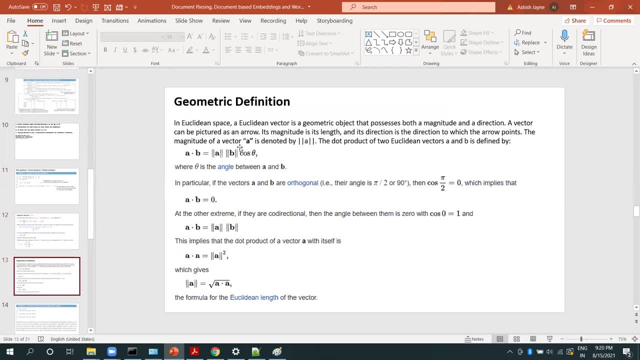 the dot product of these two, the dot product of these two vectors, then what is the geometric vectors then? what is the geometric vectors? then what is the geometric definition? geometric definition is definition. geometric definition is definition. geometric definition is simply a dot, p meaning mod of, a mod of. 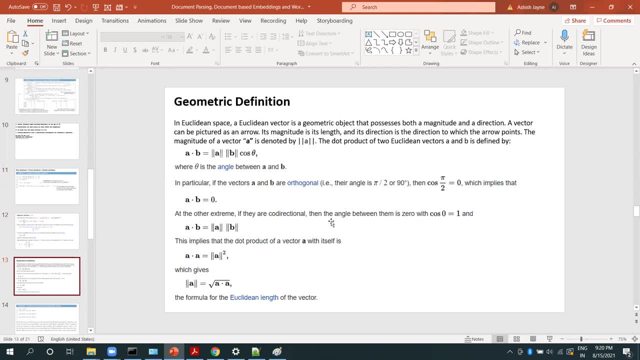 simply a dot p meaning mod of a mod of, simply a dot p meaning mod of a mod of b and cos theta, cos theta is b and cos theta, cos theta is b and cos theta, cos theta is anti uh clockwise direction, anti uh, clockwise direction, anti uh clockwise direction you take. theta angle is taken in. 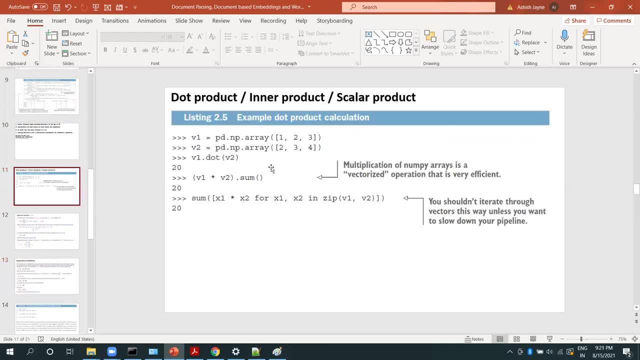 you take theta angle is taken in. you take theta angle is taken in anti-clockwise direction, anti-clockwise direction, anti-clockwise direction. now, if you have now, if you have now, if you have, this is for understanding that, if you, this is for understanding that, if you. 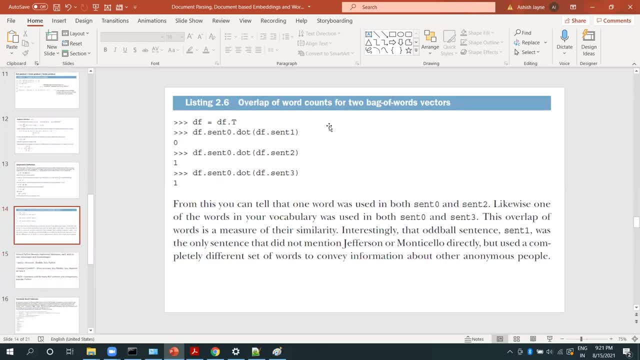 this is for understanding that if you have common words which is present over, have common words which is present over, have common words which is present over here. overlap of word counts for two bag here. overlap of word counts for two bag here. overlap of word counts for two bag of words. 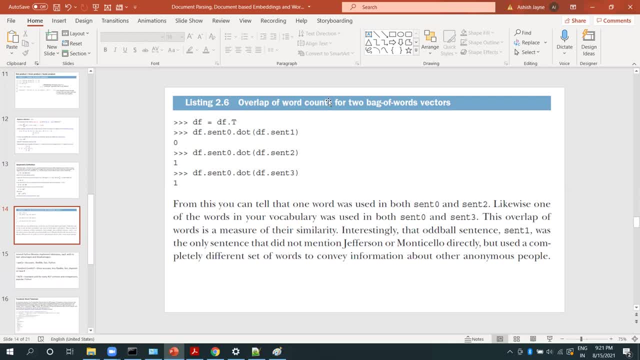 of words, of words, vectors. so if you uh do it, vectors. so if you uh do it, vectors. so if you uh do it. shall we do it as an example? let's do. shall we do it as an example? let's do. shall we do it as an example? let's do it as an example. 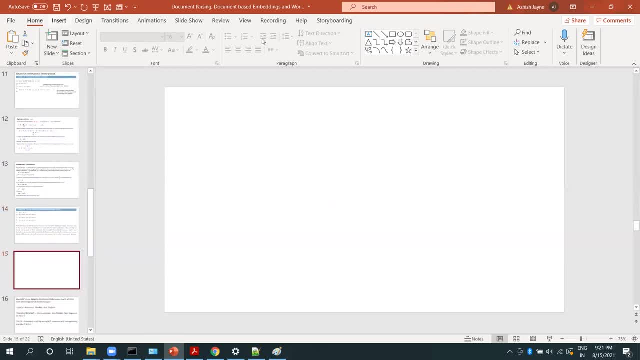 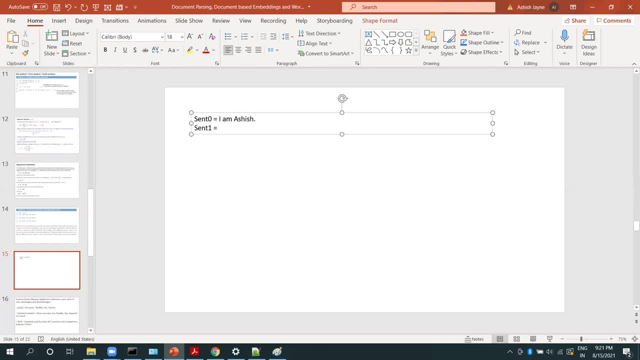 ashish, ashish, and send one equals to, and send one equals to, and send one equals to. maybe, maybe, maybe, um, not, um, not, um, not, so, uh, how many, so, uh, how many so, uh, how many? we would not sort them. we would not sort them. we would not sort them, we would simply. 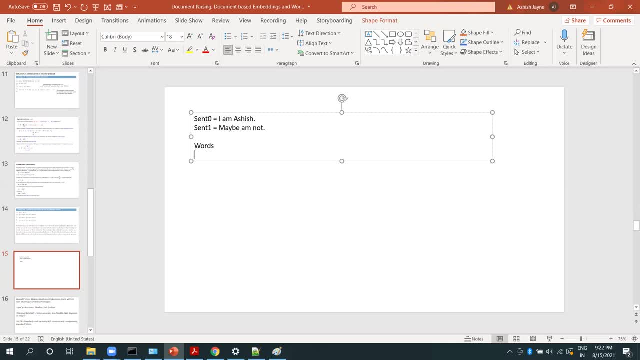 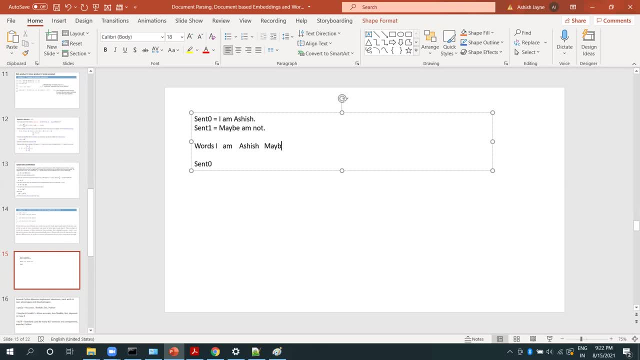 um, do you understand, or shall i need to explain this? it's fine, i'll be able to understand. okay, just a second. then sentence zero: i am ashish, maybe i'm not. i is there in sentence zero. so one zero m is there, ashish is there, maybe is not there and not is not there. 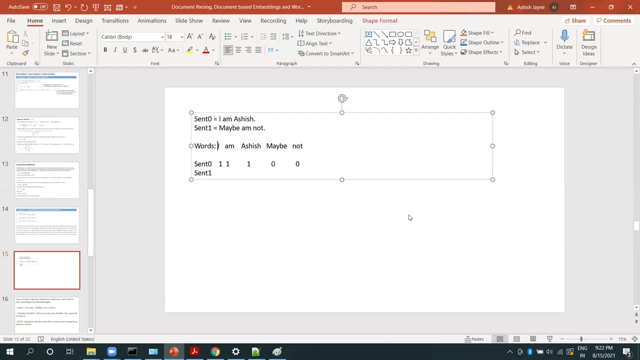 send one, then i is not there, m is there, ashish is not there, maybe is there and not. is there? now, when we dot product t2, send zero, dot send one. you the vectors, as per the definition of vectors, we have to multiply this number by this number. 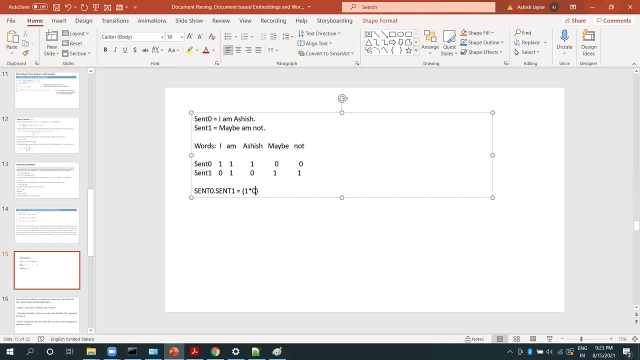 so one times zero plus one times one plus one times zero, plus zero times one plus zero times one. now this gives you essentially one, because there are zeros in the rest of the figures. when one times one is one, a number of common words. number of common words in these two sentences is one. 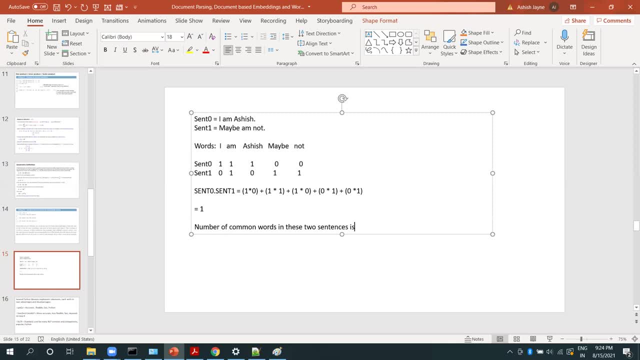 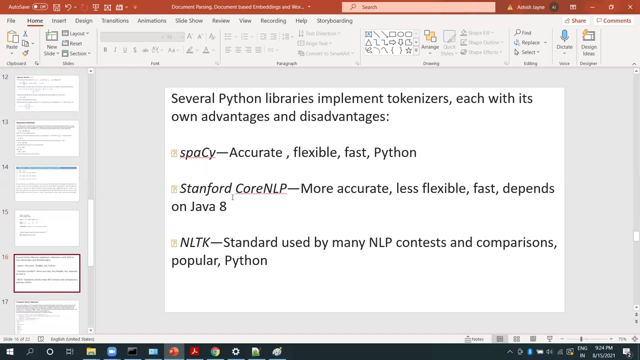 the two sentences is one an application of dot product. now, if we go to the next slide, several python packages. we come into the application point of view. like what do we have? we have several python packages implement tokenizers, each with its own advantages. you have- you must have heard of spacey nltk and 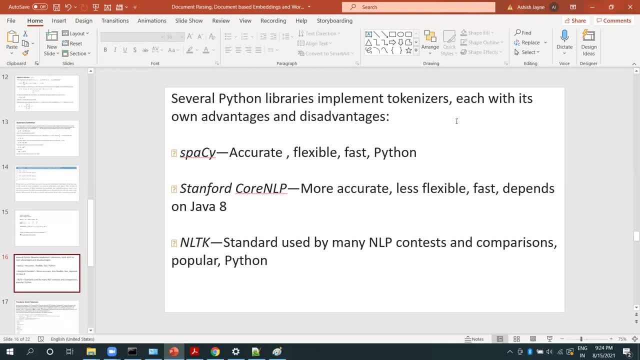 stanford core nlp. you must have heard of spacey nltk and stanford core nlp and stanford core nlp. spacey is the industry standard for doing basic tasks such as tokenization but a tokenization, but otherwise nlp is also a very good package. stanford core nlp i have personally. 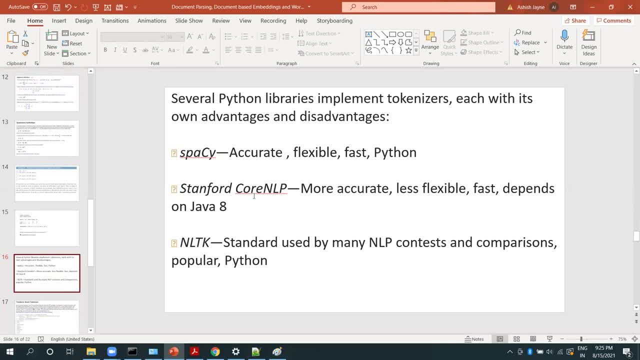 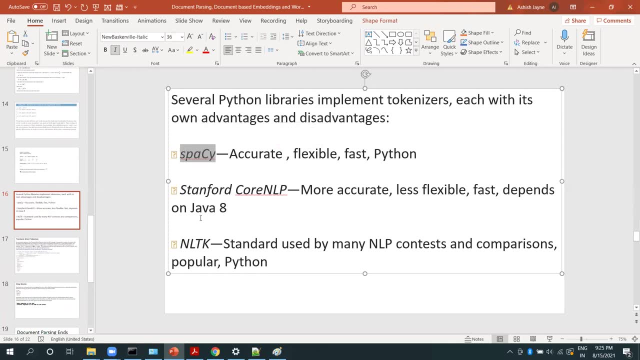 not used this, as it uses java and most of uh the work that i have done is in python and it's good to remember these two packages for now, as most of our examples are in python and this book is also written in python now. the end of this webinar will be commencing in a 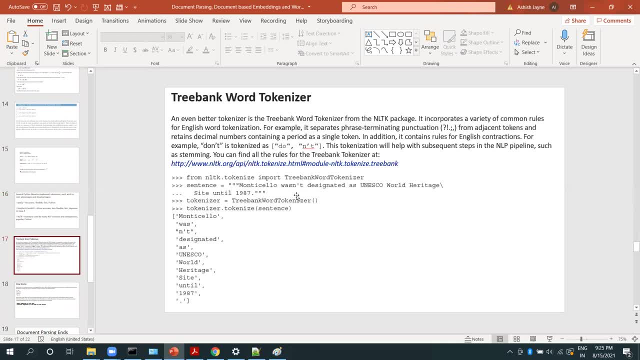 so long, till the end or начала. bye, bye to you in the next class. bye bye, ciao. see Now TreeBankWorldTokenizer. this is a tokenizer that's available in the NLTK package, and this is a piece of code that is explaining you how to use it. 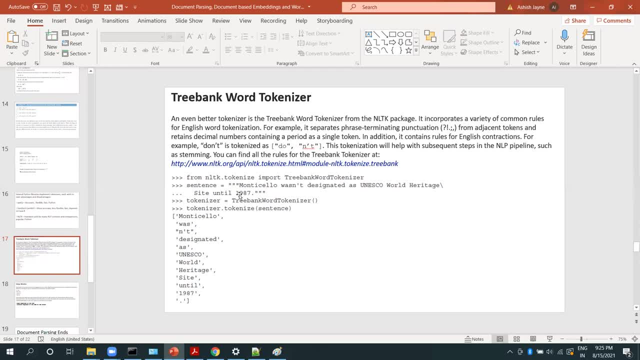 You do the import, you create an input sentence, you initialize the tokenizer variable by calling the constructor for that TreeBankWorldTokenizer class, and then you use the tokenize method of tokenizer to tokenize a sentence. Now, as you can see, this TreeBankTokenizer has been trained to understand contractions. 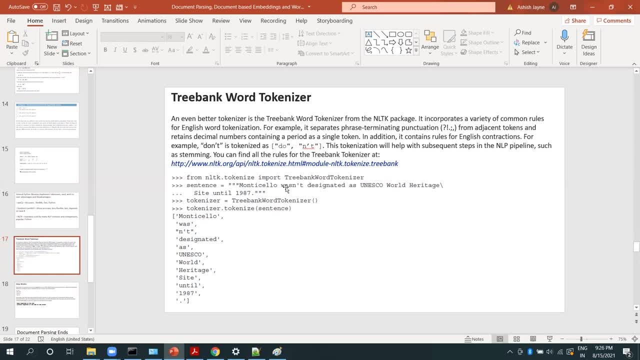 as well. What are contractions? The words such as wasn't, don't their, there, isn't they t-h-e-y, apostrophe r-e. it's able to understand them and break them into separate words, such as if we have a sentence. 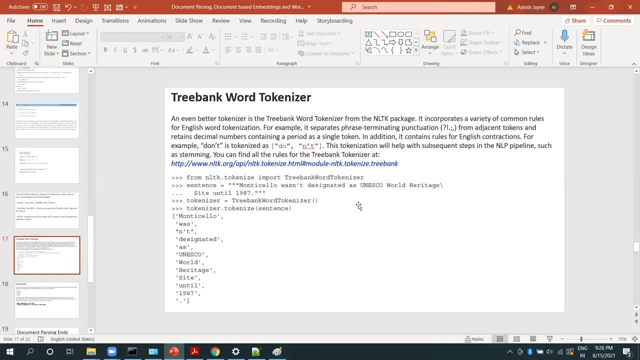 Monticello wasn't Designed as UNESCO World Heritage Site until 1987, this word wasn't has been broken into two, was and not, not, not exactly not, but an N apostrophe T, So TreeBankWorldTokenizer is a pretty good one. 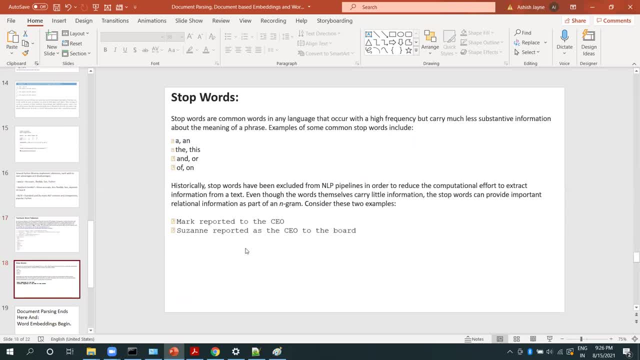 You can use it in your projects. Stop words: What are stop words? These words are, basically, which are extensively used in your English language writing and you can ignore- Safely ignore- them for your NLP application. Now, at times it is not advised that you remove stop words such as the word not because it. 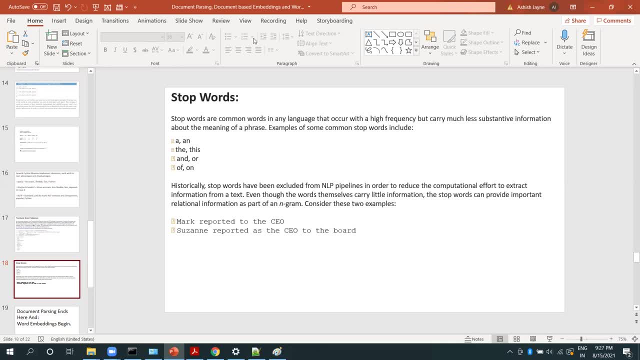 changes the meaning of the sentence, such as in the problem of sentiment analysis. What happens is that if you tell the sentiment analyzer I am happy and you use the stop words removal to remove I am, then only happy is left, Happy is past. 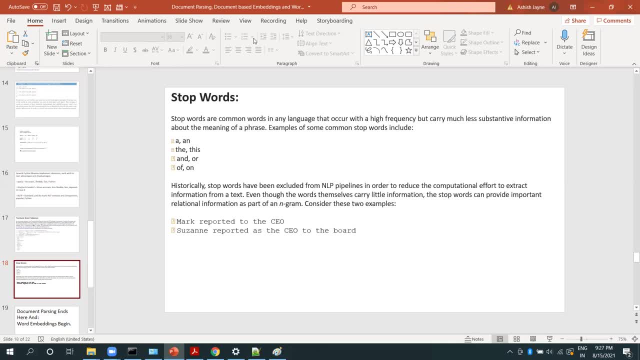 Happy will be left. The rest of the sentence is positive. Happy is not a positive sentence because there are some negative things in it. As you can see, I am not happy Now if you have a stop word removal library which is also going to remove the words such 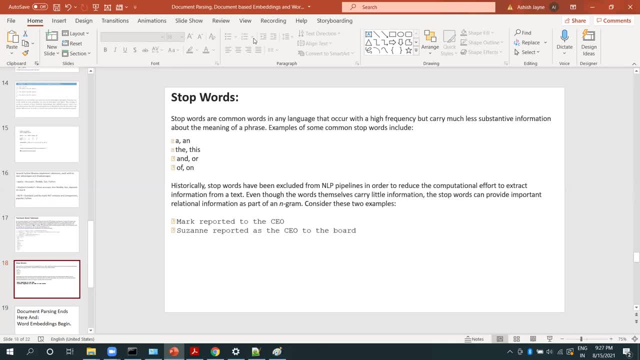 as not going to remove the words such as not, then that will create a problem, Because if you're using stop words and removal and the input sentences I am not happy sentence Stop words removal will remove I am not and only happy will be left, which will result in the wrong output of positive. 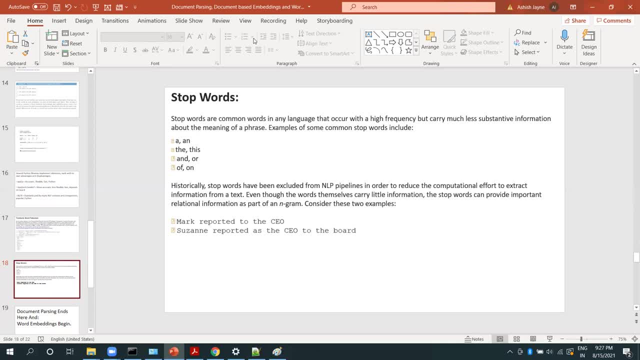 or positive. Let's move on. So I have two choices here. The first choice is that I have only happy, Then I will remove happy. The second choice is that I will. Do you want to use the word or not? Okay, I will. 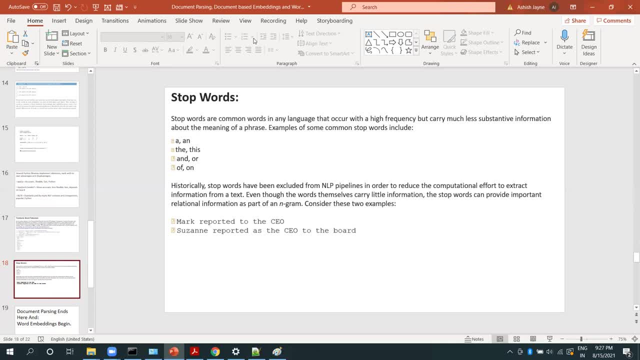 positive sentiment. so at times, stop words removal is not a good idea because it these stop words help us figure out the relationship between the words. what relationship is present between different relation? what relationship is present between two words such as the example over shown is Mark reported to the CEO and Susan reported as a CEO? just a change of two, just a change of. 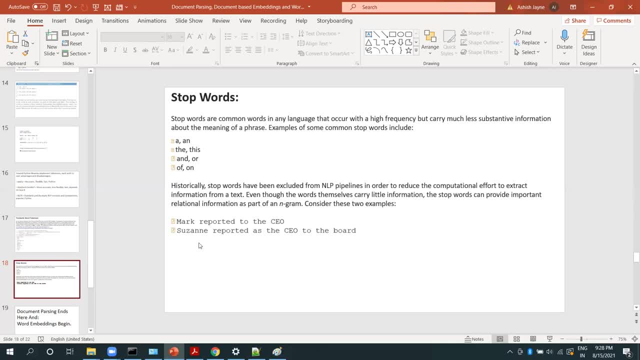 single word of two to, as which, both of which are stop words, you are essentially destroying the meaning of relation, the relation, the all the context of relationship that Mark and Susan have with the office person CEO. now Susan is the CEO, CO is the reportee, but if we remove the stop words, it both becomes mark reported, the ceo sort of d. 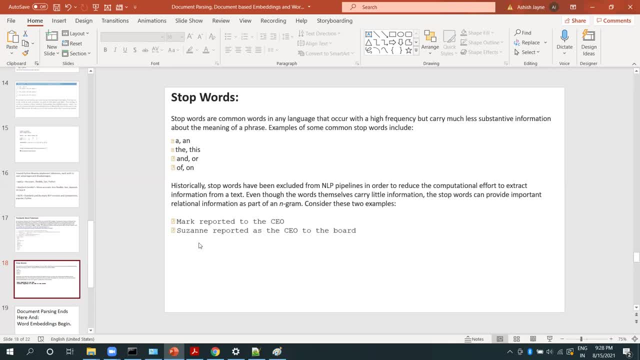 will also be removed: mark reported ceo. and for susan it will be susan reported ceo. so this is kind of becoming. we are losing the relational information in the text by removing the stop words now. next is word embeddings. now word embeddings, document parsing ends here and word. 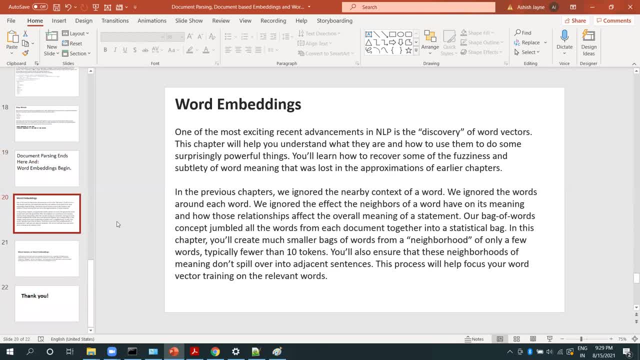 embeddings begin. we don't have too much content for word embedding right now, but all that you need to understand is that computers work with numbers. at the most basic level, they work with zeros and ones, and to make your text understandable to a computer, you have to turn it into some kind 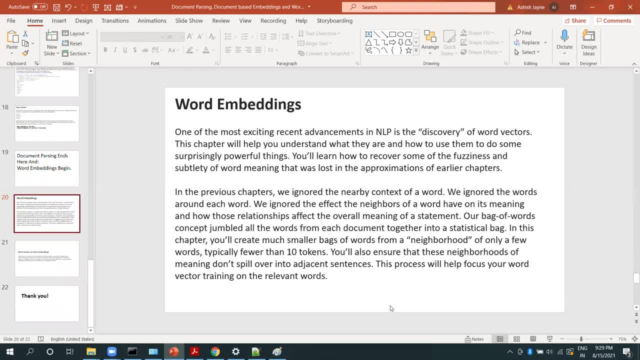 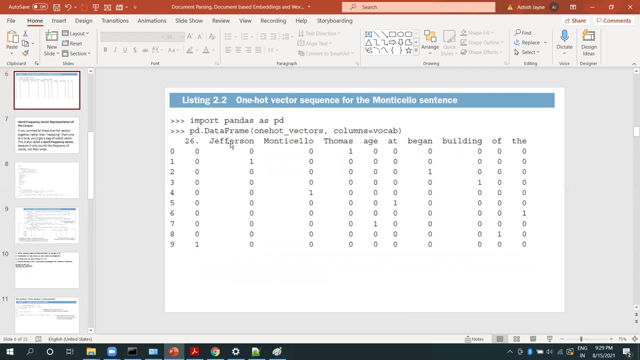 of numbers and those numbers are called word embeddings. now there are some word embeddings which are local, some are global, but once again, if we have that here i would not okay. so when we talk of local word embeddings, what we saw over here, like over here, if we have some kind of text, the embedding for the jefferson. 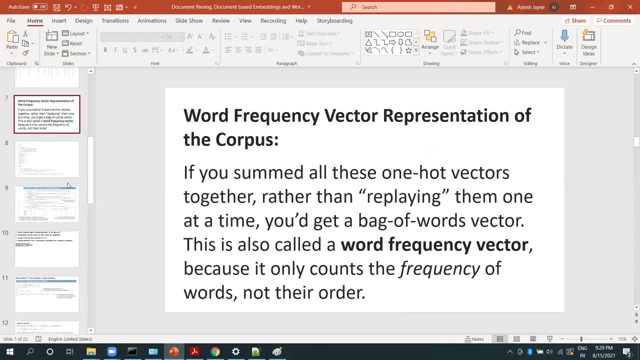 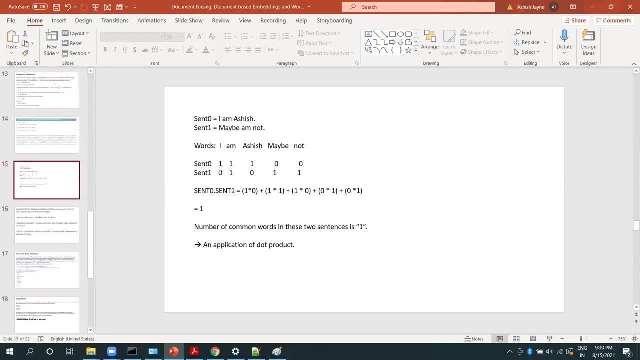 is zero, one and all zeros in the one hot vector representation. the embedding for the word embeddings is called word embeddings. now there are some word embeddings which are local, so i think the word embeddings concept is a bit confusing because i would need to figure out how the word embeddings concept comes there. but basically it is the representation of the. 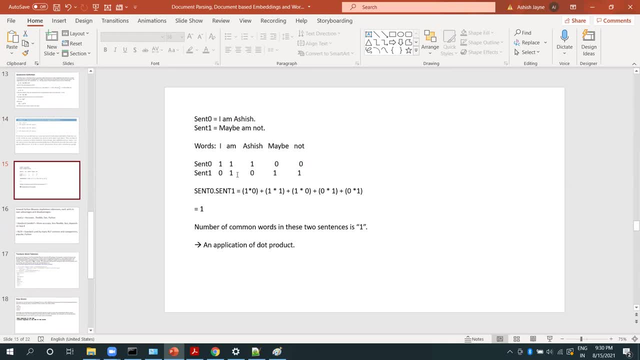 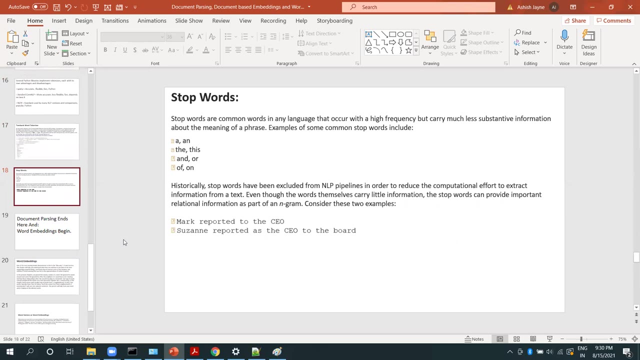 document and not the words. but when we do something like this, we are essentially converting our corporas, our input, into numbers that are understandable to the documents, and we have a lot of information in the document. and we have a lot of information in the document: the concept of local word embeddings and global word embeddings. now, when we talk of local word, 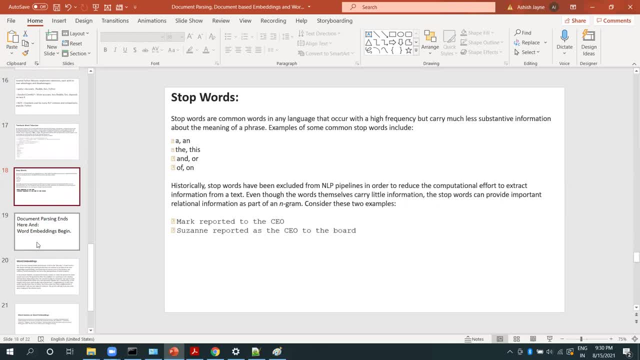 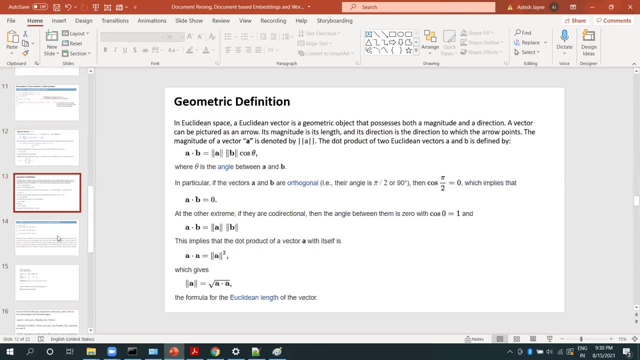 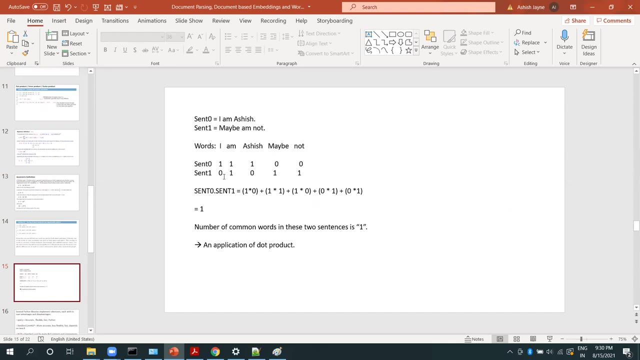 embeddings. they are created by count vectors such as this: count one second um. count vectors- number of times it appears in the document. uh, count vectorizer, so i. there is a concept called count vectorization which should be able to return the word local word embedding for these words with respect to sentence zero and sentence one. but we also have a concept called 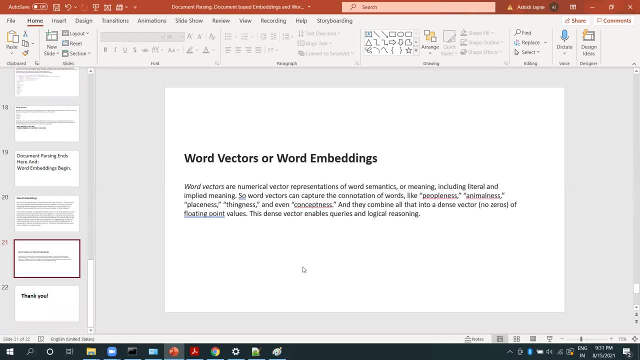 global word embeddings, which are which essentially take the name of glove, or word2vec, or bird embeddings. but to begin with, to conclude this session on on one line, global word embeddings, uh are fixed length embeddings that know what a word is and they understand the word in terms of its. 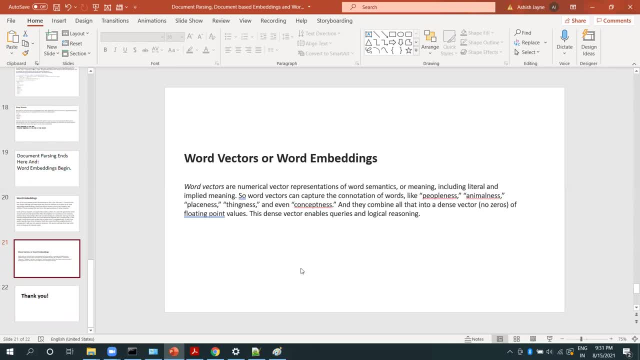 features such that, such as its gender. what is the gender of the word? animalness of the word, peopleness of the word, if the word is the name of a place or a thing, or even if it is a concept. for example, if a word embedding bird understands. 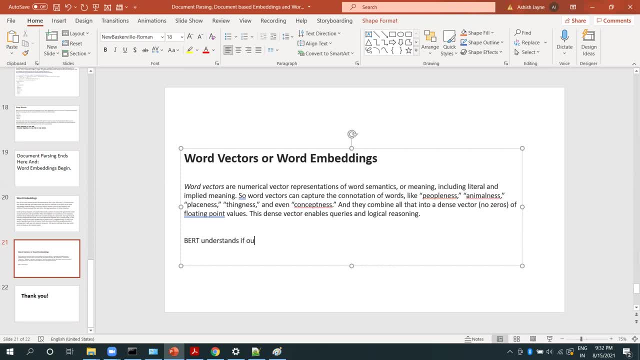 whether if if word understands, if you uh talk to it, talk to it about python, word would understand whether you were talking about a reptile, talking about a reptile or not a reptile, but the animal, the snake, the snake or the or or the lab programming language. so concept is also. 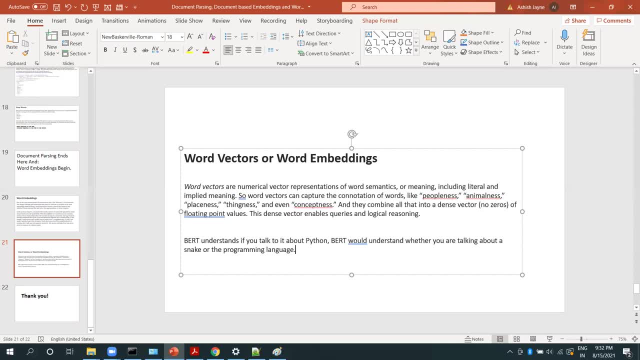 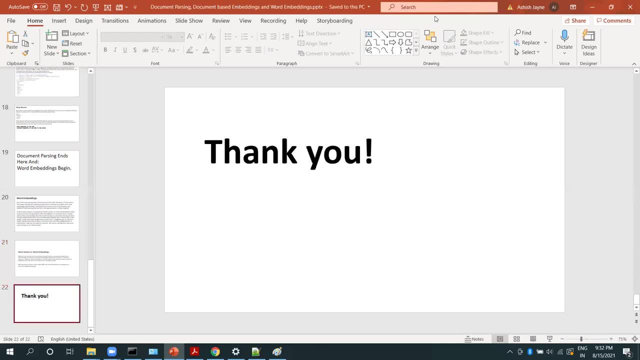 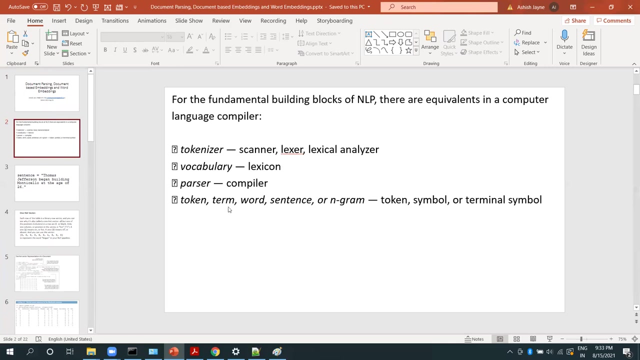 captured by global word embeddings. so this was all for today. thank you for joining any questions, any questions you have. uh, any questions? um, no questions, an sh. but there was a term in one of the slides: n gram. okay, and yeah, this one, i think. okay, n grams. so when we call n gram, it is we basically mean two gram or three gram. 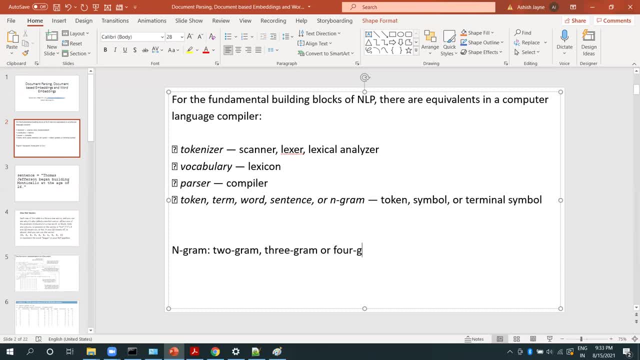 or four gram, and, or, and so on and so forth, so on, right in two gram, meaning we have to take out words together, like if we have the sentence, this sentence, and we will copy it here. when we have a tokenizer that is picking out, it will pick out thomas jefferson.